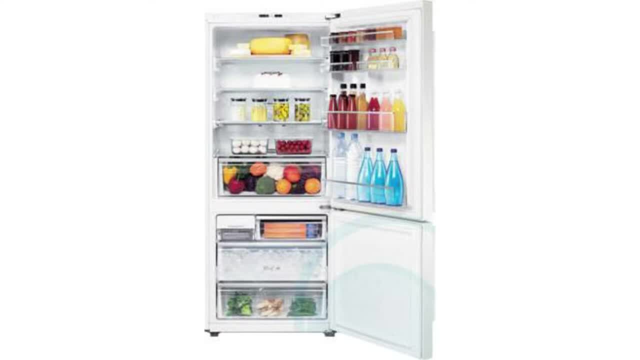 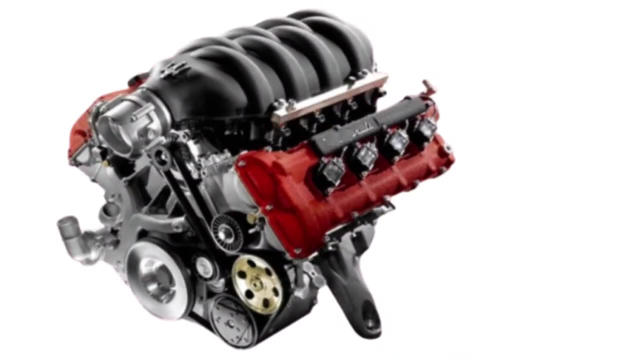 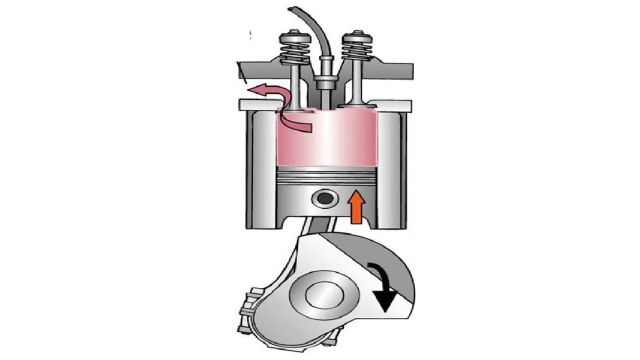 in detail. Okay, what's happened in the refrigerator? So refrigerator is my system, Same like as in IC engine. my study is: what is the behavior of combustion in IC engine? So at that time, the engine is my system, So we can consider any part of universe as a system. Okay, system is separated by boundary. 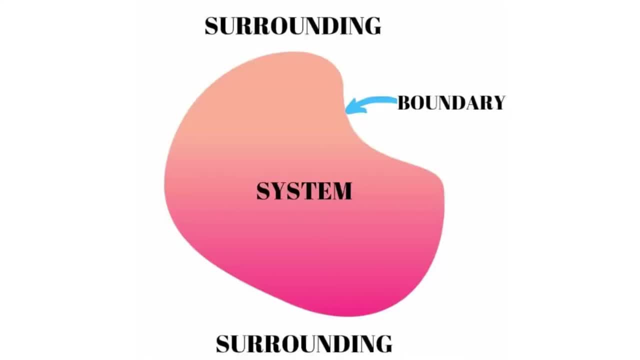 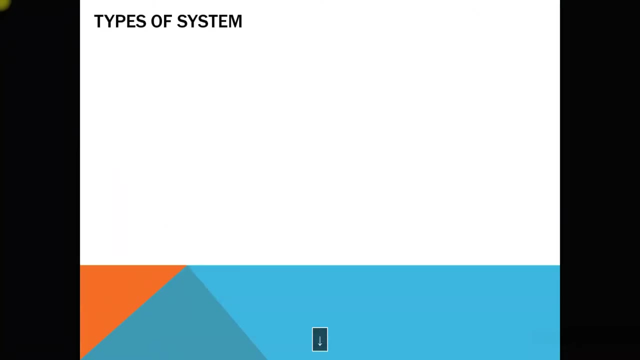 from the surrounding. So boundary means it will separate the system, and surrounding It is called boundary, and surrounding means outside the boundary. Now we will discuss types of system. The first one is open system. In open system there is a transfer of mass. 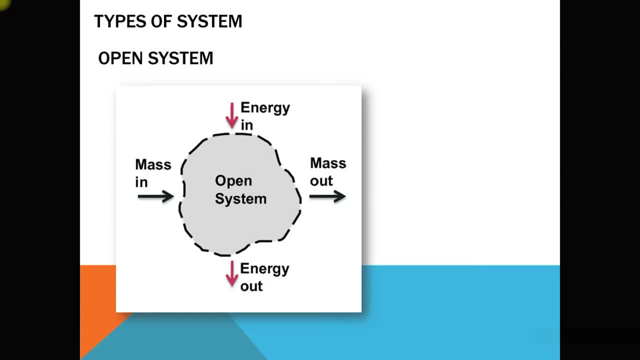 as well as transfer of energy. So in case of open system, mass and energy, both are crosses the boundary. It is called open system. Let us take one example of a vessel: Okay, and this vessel is heated by some external source, like as coal. we can say any burner Okay. so whenever we supply, 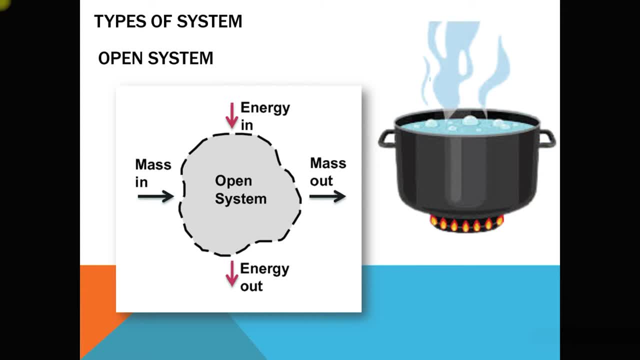 the heat to any open vessel. water is filled inside the vessel And whenever we supply the heat energy at that time, this water will start to boil. Okay, so at that time, what's happened? there is a transfer of heat as well as transfer. 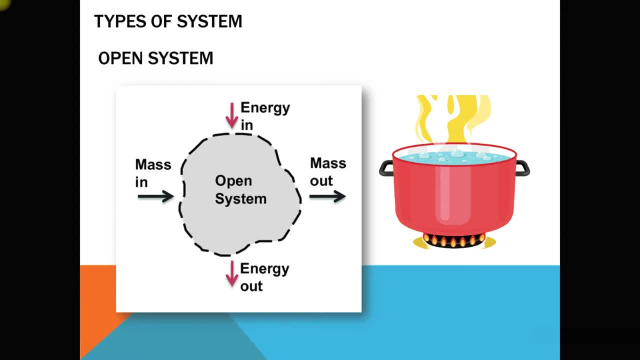 of mass, Because this vessel is open and it will start to evaporate and whatever the steam it will be generated, it is transferred to atmosphere, It is transferred to surrounding. So it is the example of open system. So in open system there is a transfer of mass as well as transfer of energy. it is called 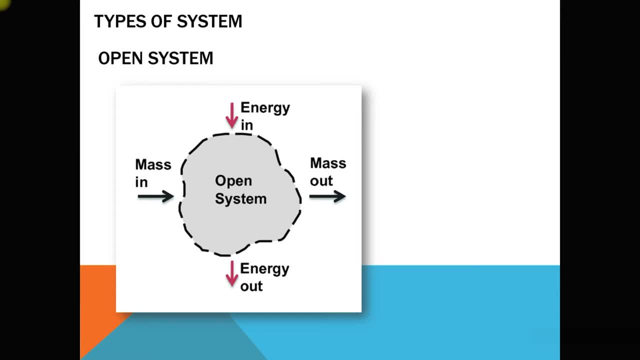 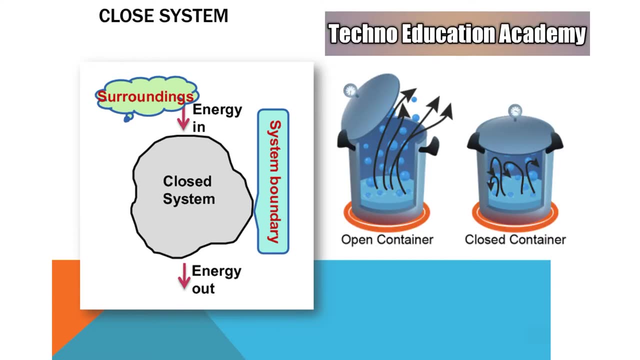 open system, The next one is closed system. Same example here we are considering, but except that here we are considering the vessel is closed at top side, So there is no any transfer of mass. So whenever we supply the heat energy, this heat energy, it is stored as a internal energy. 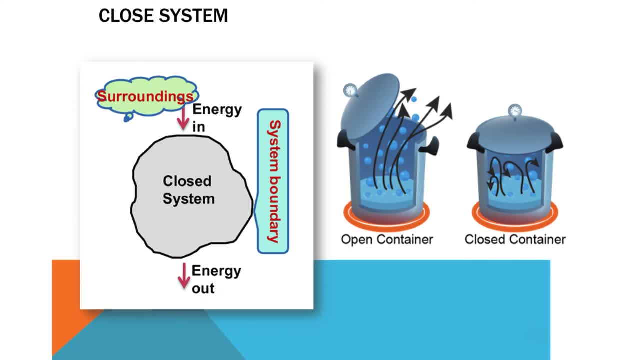 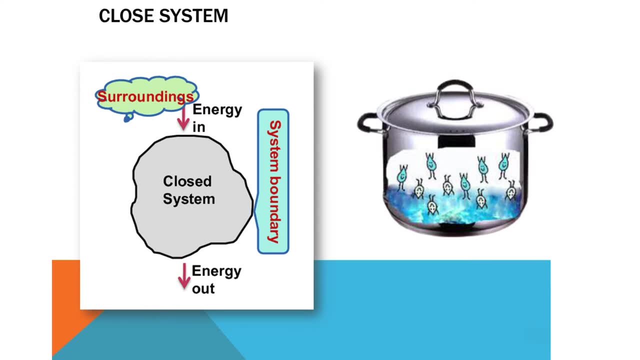 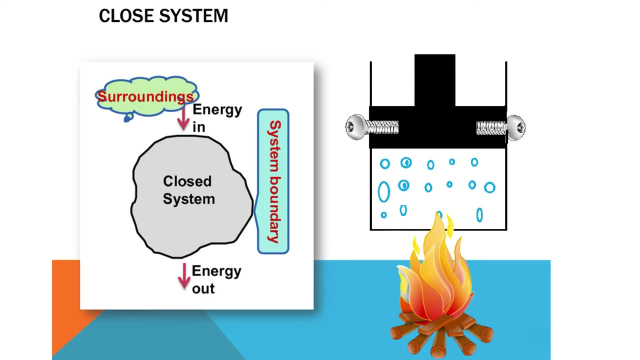 and there is a transfer of heat to the system, But there is no any transfer of mass, because here we are considering, the vessel is closed at top side. We can also consider the example of a vessel. In a vessel the piston is fixed by some locking device or we can say some fixture or screw. 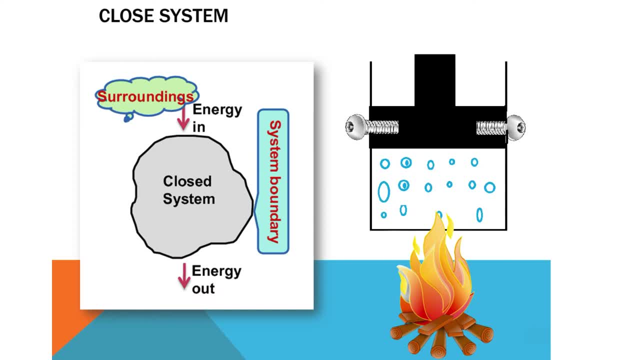 So there is no any movement of piston and it is filled with air At bottom side. we supply the heat energy by any of the external forces. So whenever we supply the heat energy, so this heat will be transferred to the vessel and there is a molecular motion will be there inside the air particles and the internal. 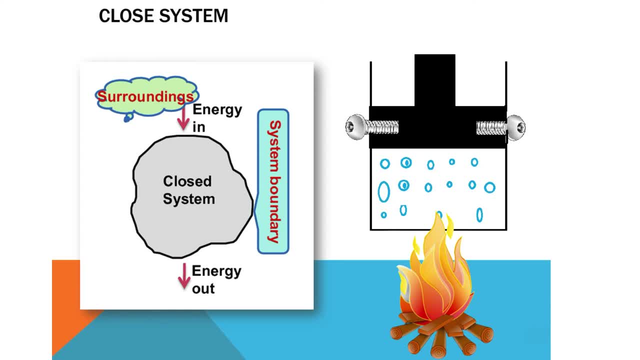 energy of the system will be changes. So here the piston is fixed, so there is no any transfer of mass to the surrounding, But here the heat transfer will be there. So we can also consider the example, For example, of closed vessel. it is fixed with piston, with some locking device. 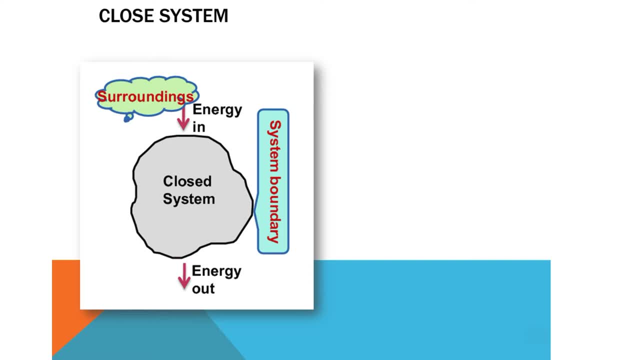 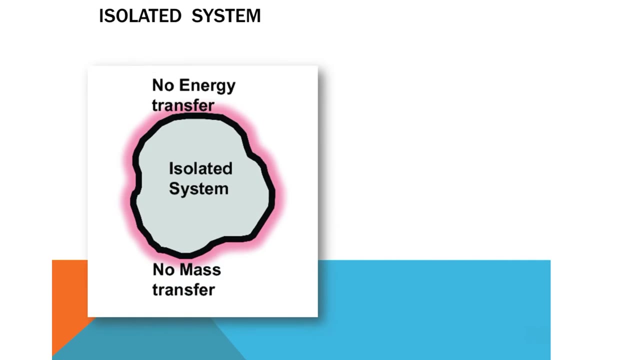 So here there is a transfer of heat, but there is no any transfer of mass. it is called closed system. The next one is isolated system. So in a isolated system there is no any transfer of mass as well as there is no any transfer of heat. it is called isolated system. 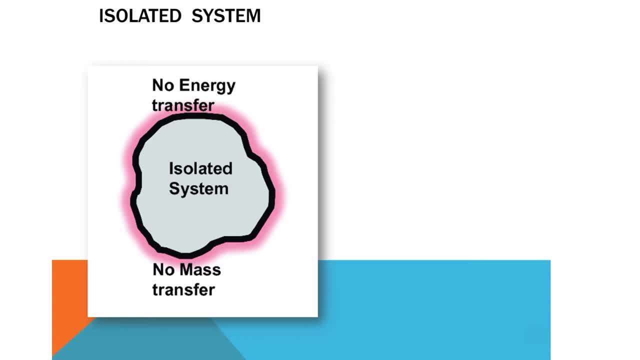 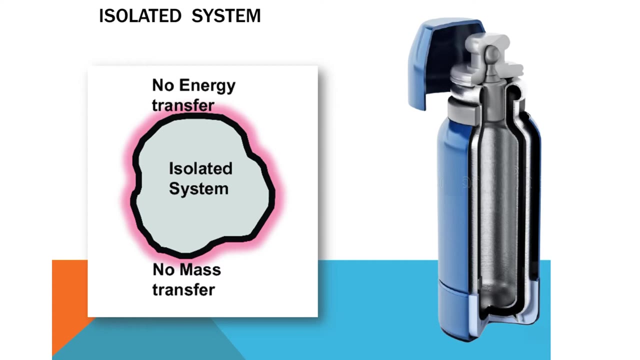 So here mass and energy, both are not crosses the boundary. In practical life there is no any isolated system. but we can consider the example of thermos. So in thermos there is no any transfer of mass, as well as there is no any transfer of. 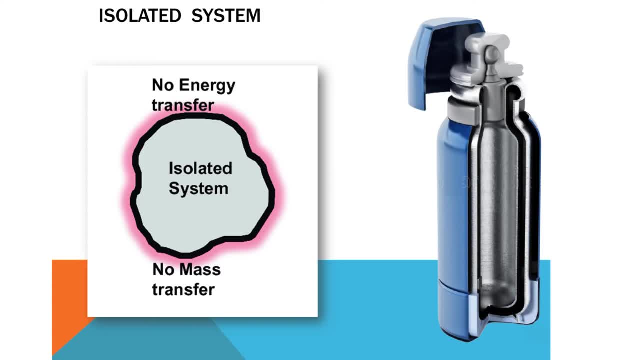 heat. So whatever the fluid is filled inside the thermos- either it is a hot fluid or cold fluid- It will maintain its temperature for a long time. So in a isolated system, there is no any transfer of mass, as well as there is no any transfer. 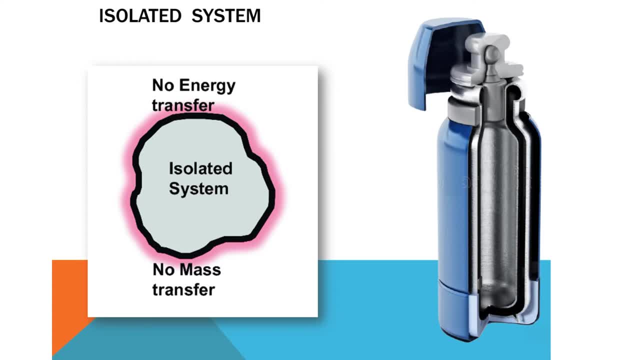 of heat. So whatever the fluid is filled inside the thermos- either it is a hot fluid or cold fluid- It will maintain its temperature for a long time, Because we know that the construction of the thermos: it is made by two layers and between, 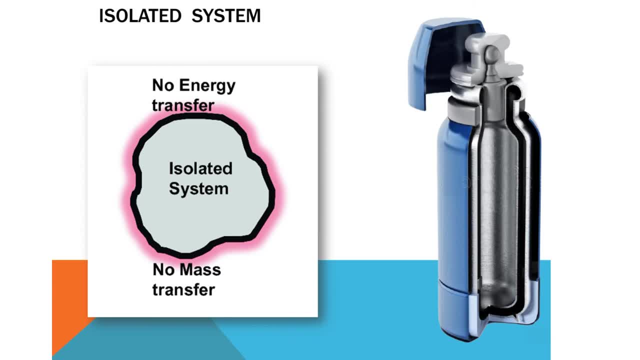 the two layers there is a vacuum. We know that vacuum means pressure below atmospheric pressure or we can say there is no any air inside this pass and we know that air is responsible for convection. So whenever we provide the vacuum In a thermos, so we prevent the heat loss due to convection as well as for conduction, we 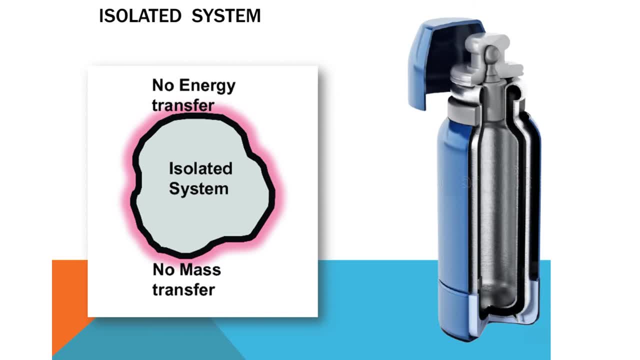 required the medium. So there is no any physical contact. So conduction is also we can prevent. So we can also prevent the conduction. and we know that for radiation there is no any medium is required to transfer the heat. So inside the layer of the thermos. 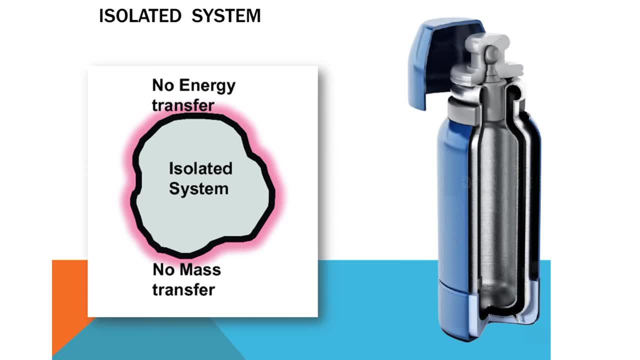 So we are also providing the reflector, and the function of the reflector is to reflect the radiation. So for a long time we can store the hot fluid as well as cold fluid and we can maintain the temperature for a 6 to 7 hour, or we can say 8 hour. 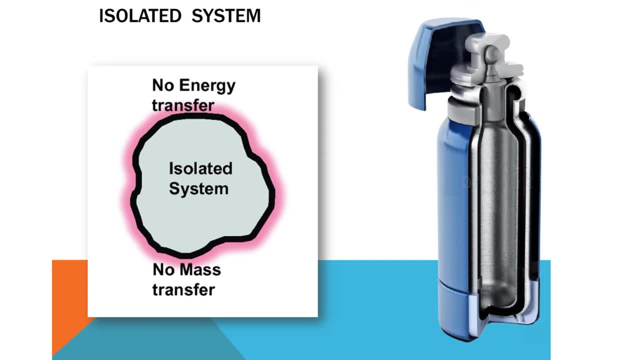 So we can consider the example of thermos as a isolated system. So in isolated system, there is no any transfer of mass, as well as there is no any transfer of heat. So let us see, So, let us see, So, let us see. 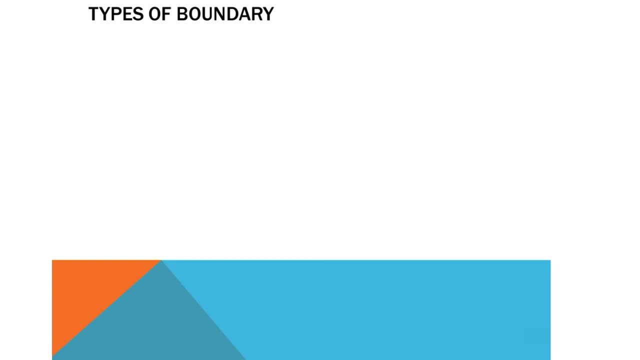 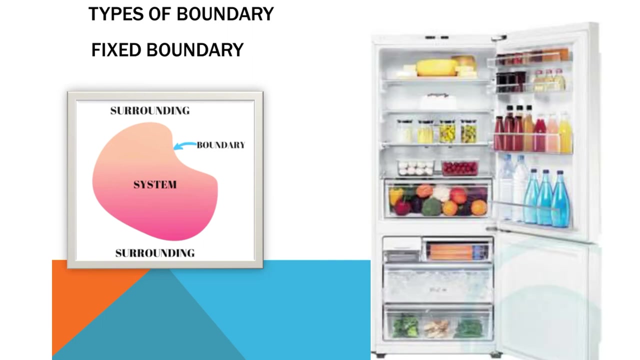 We have already discussed boundary means it will separate the system from surrounding. Basically, there are three types of boundary: fixed boundary, movable boundary and imaginary boundary. Fixed boundary means boundary does not change with respect to any external parameter, For example, whenever we consider the example of refrigerator body. ok, it is the example. 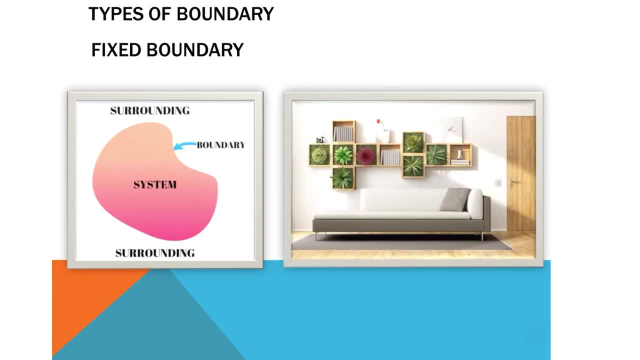 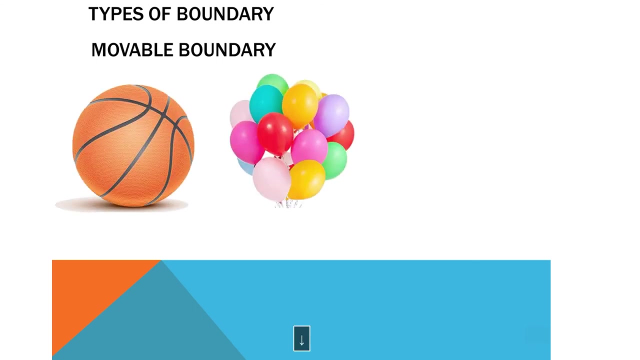 of fixed boundary. We can also consider the example of a wall: ok. The example of engine body: ok. these are the example of fixed boundary. There are so many example we can consider as a fixed boundary: IC engine ok. pressure vessel ok. So fixed boundary means boundary does not change. 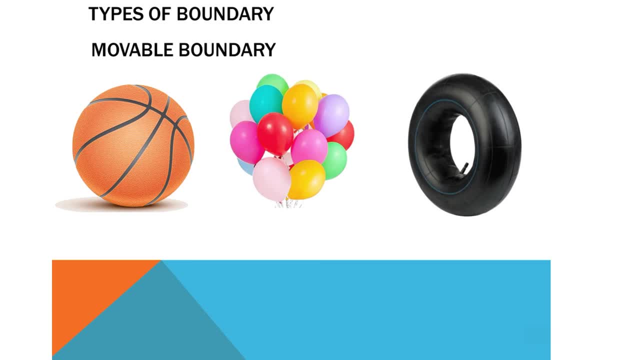 The next one is movable boundary. So in movable boundary boundary will change. ok, for example, in case of a balloon. ok, whenever we fill up the pressure or whenever we inflate the balloon. ok, at that time it boundary will change. it is called movable boundary.